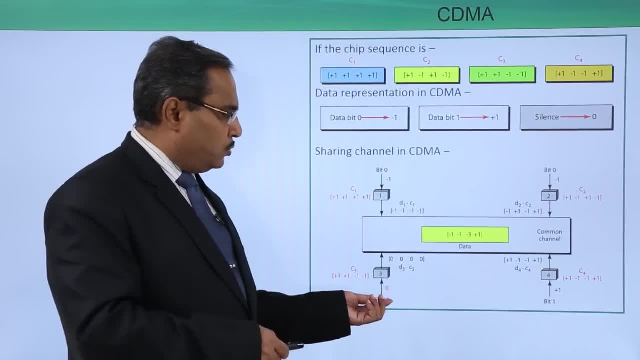 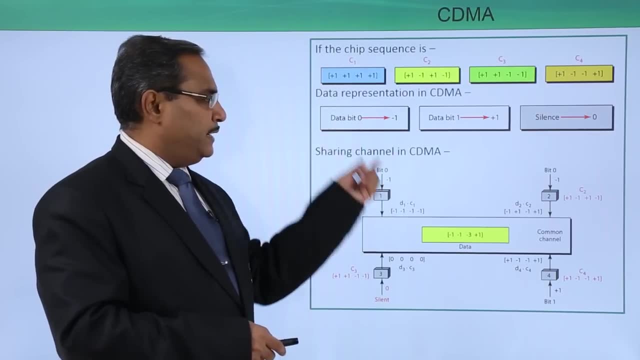 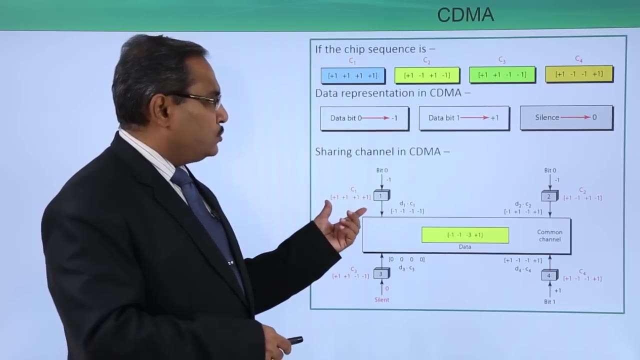 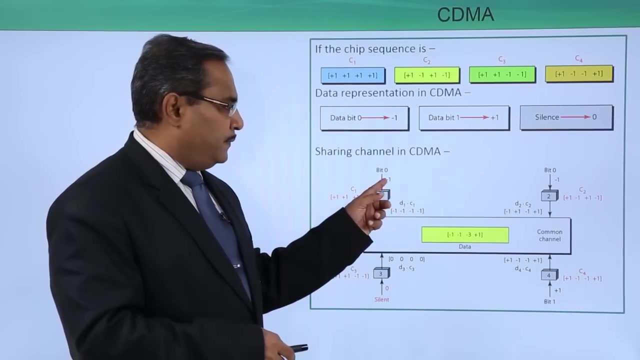 So now, this is the silent node and other three nodes are transmitting Good. It is transmitting minus 1.. Means what It is transmitting: data bit 0.. It is transmitting minus 1.. It is transmitting plus 1.. Means what Data? bit 1.. So the codes we have written, these are the respective codes We have written that one across the nodes in different color. Now see, this is the D1, this is the C1.. Now go on multiplying, So all the signs are the same. 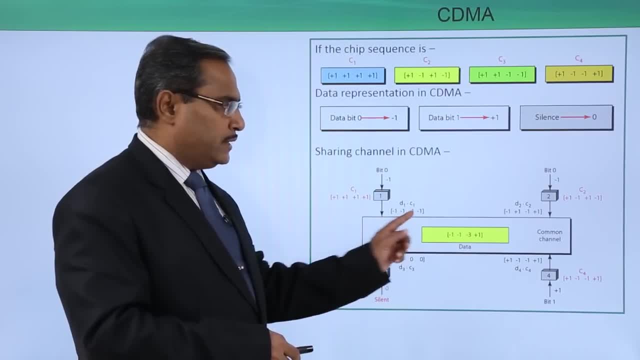 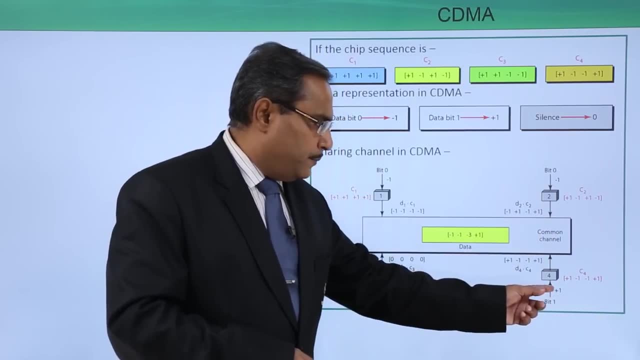 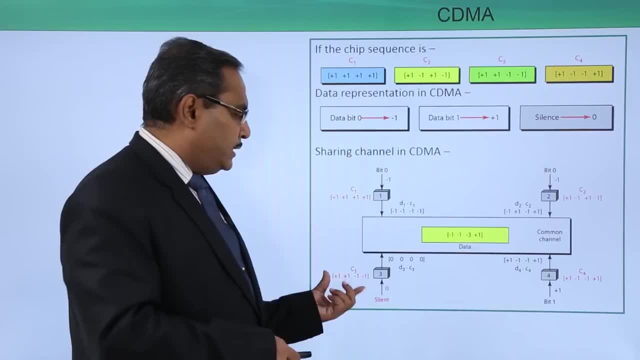 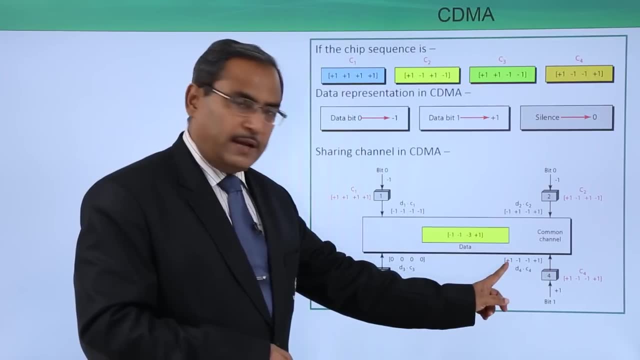 1 into this. So these are respective. And 0 into this. these are respective 1.. Now go on adding Minus 1, minus 1, minus 2, plus 1, minus 1, plus 0.. So minus 1.. So 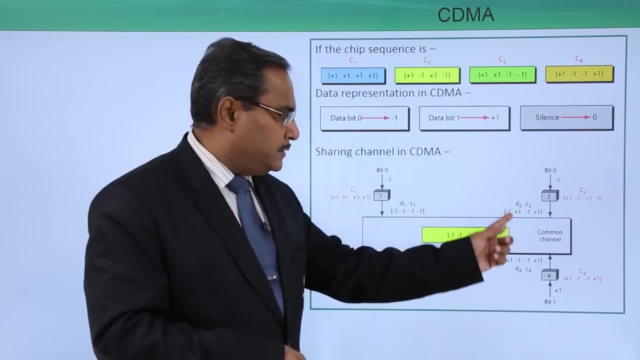 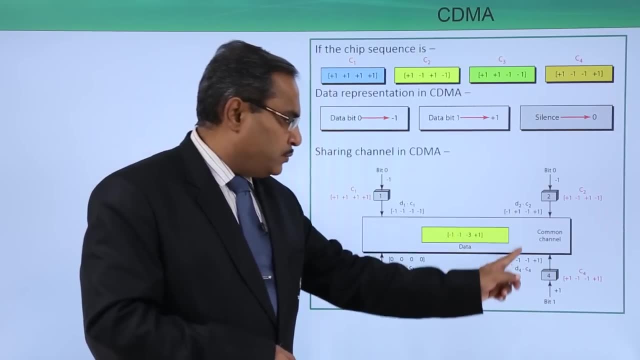 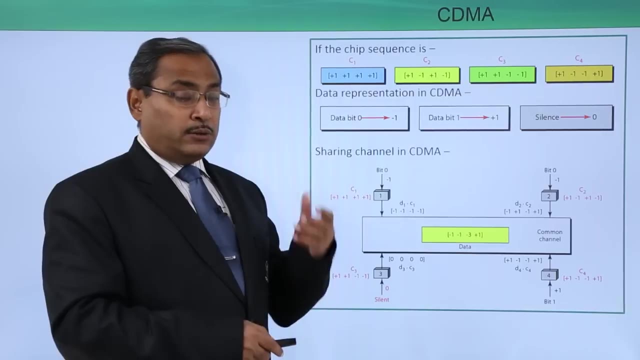 let me go for another one. So minus 1, plus 1, 0.. minus 1, minus 1, 0. ultimately, that is minus 1 if you go on adding minus 1, minus 1, minus 1, 0.. So minus 3. in this way, the respective data will be sent to the common channel. 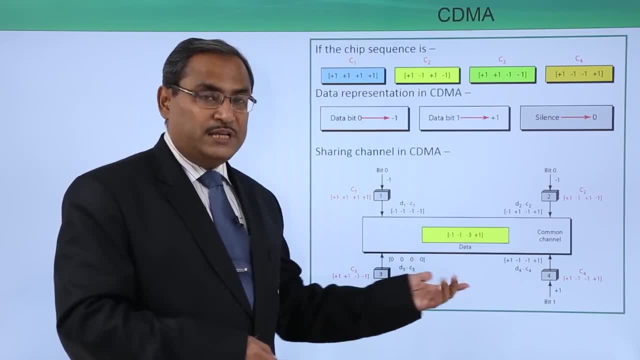 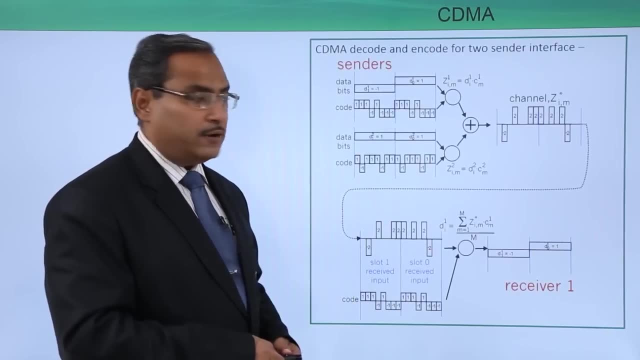 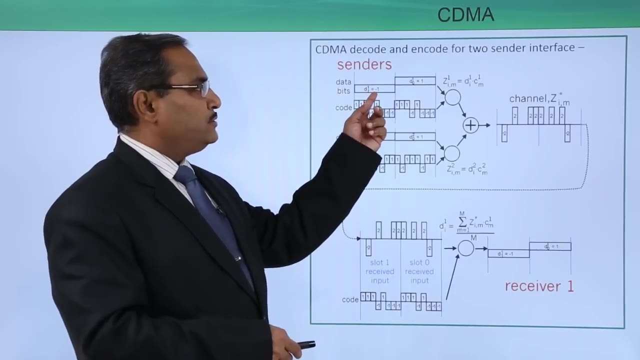 Now the question is now in our mind, then, how this particular data will be decoded. So now let me go for another diagram. I think that will be better for us. So here we are having 2 senders, say sender 1 and sender 2. it is trying to send this minus 1 and this. 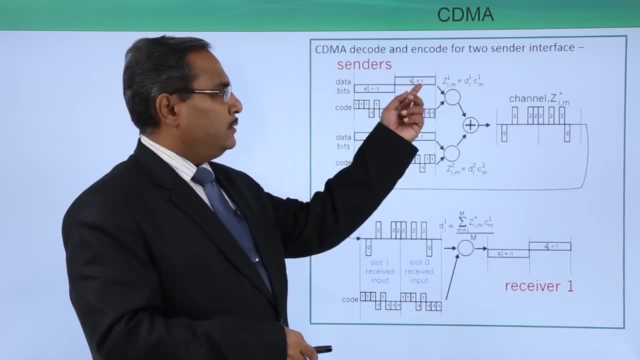 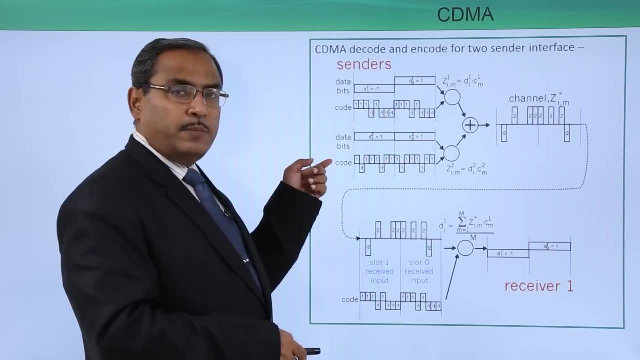 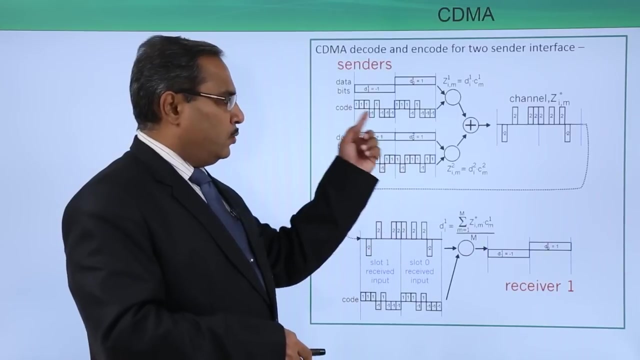 is the respective code. it is trying to send plus 1. it is the respective code and at first it is sending this one, then it is sending this one and this is our sender number 2, which is having this code. this is the data having this code. this is the data. codes are same. 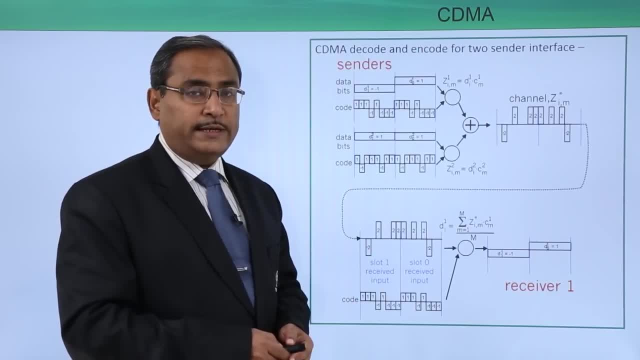 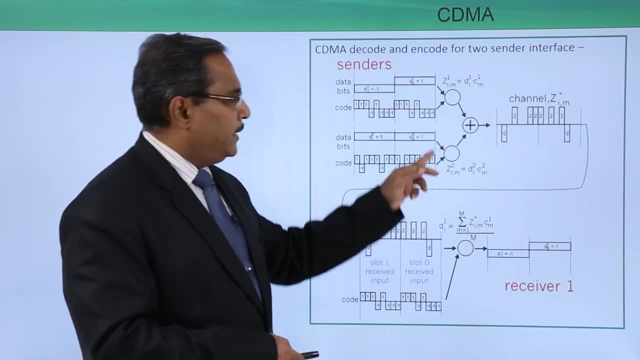 codes are same, but codes are different in this case, obviously, because all the senders will have some different codes. So now what will be the resultant here? just consider this slot number 0. just see here: 1 is there, So they will remain intact. 1 is there, So they will remain intact. So 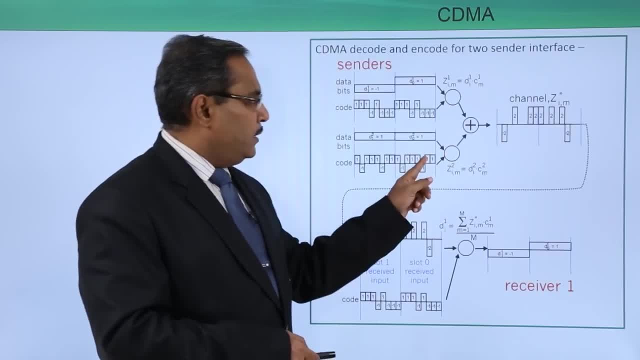 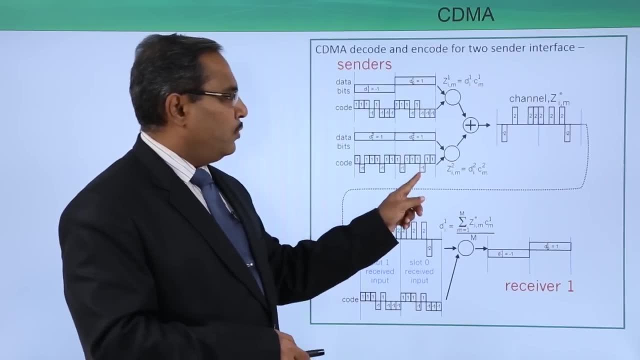 1 plus 1, 1 plus minus 1.. So that will be 0, 1 plus minus 1. that will be 0 minus 1 minus 1, that will be minus 2 if you go on adding. So 1: 1 if you go on adding, that is 2 minus. 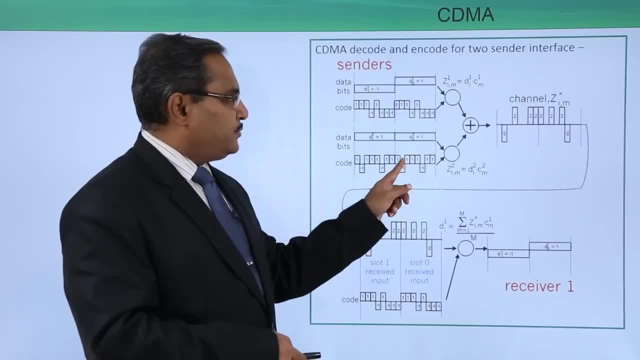 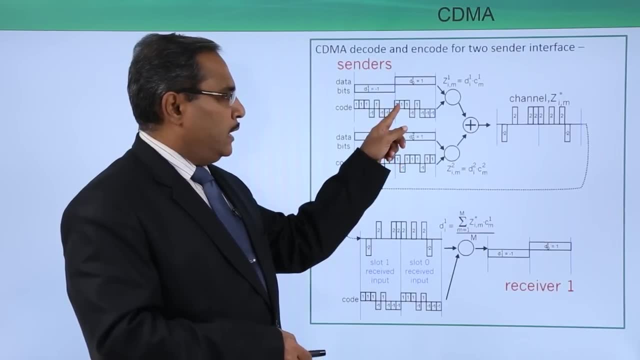 1: 1. that will be 0. I think you are getting me. Next one is 1: 1. we are getting 2. here we are getting 2, and then this is my minus 1 plus 1.. So here will be 0. this 1 is 0 and there is 1, 1 positive. 1 positive 1, if you go on. 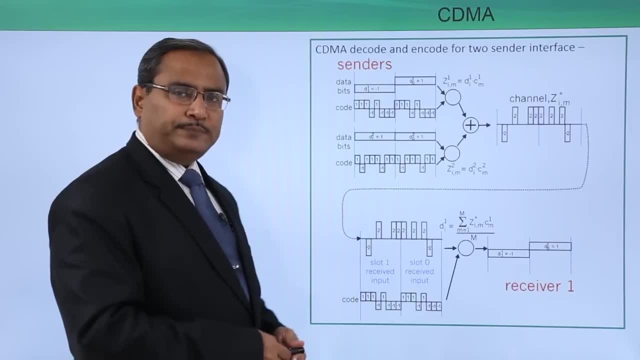 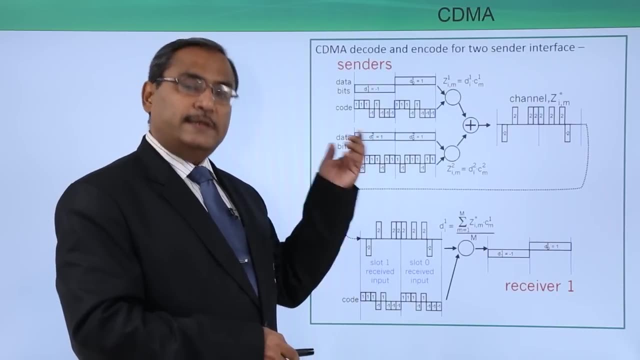 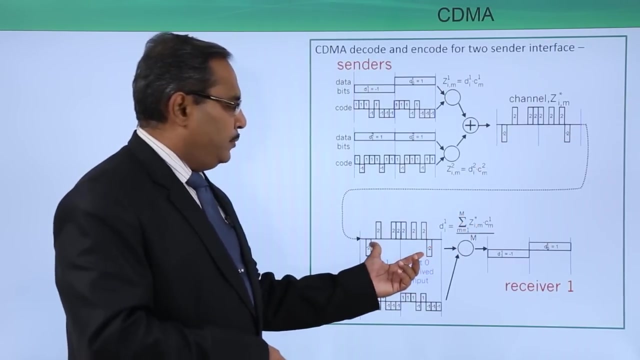 adding that will be 2. in this way also, you can calculate this one. Now let us suppose sender 1 is sending the message for the receiver 1, sender 2 for the receiver 2- just consider receiver 1 in this case. So what will happen? it will be obtained here. it will be obtained, ok. So what is this? these? 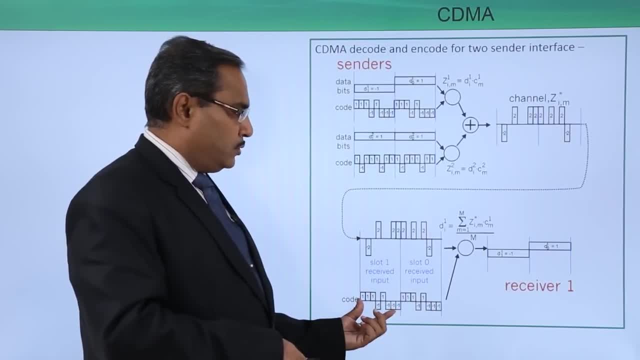 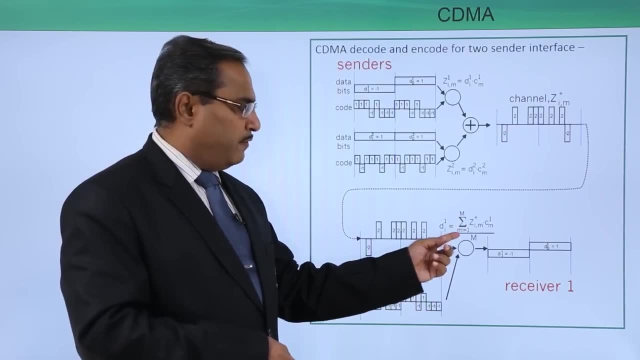 are respective sender 1's code. you see sender 1's code, Now how this receiver can get the information. what will be done? you can find we have written this one in this algebraic form, but let me go for the example. So now they will be multiplied and the sum will be. 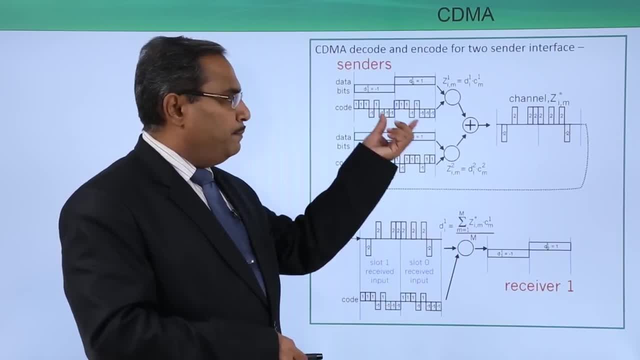 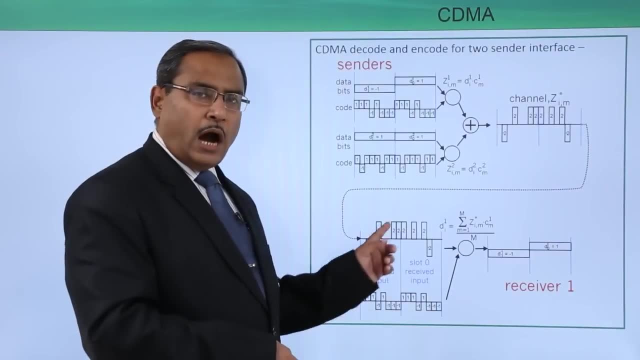 divided by this m. what is m? there is a number of bits in the code. So how many bits are there? It is 8 bits. So now let me go for the example. Now see how this receiver 1 will do the calculations. 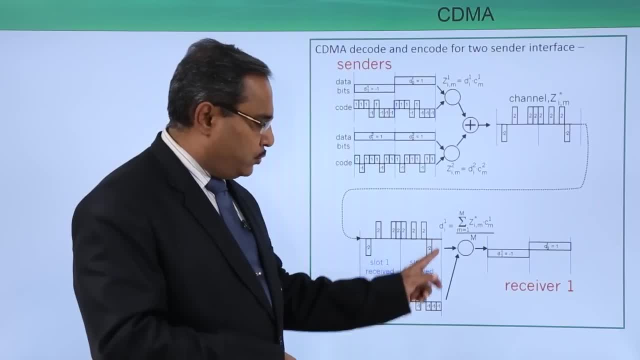 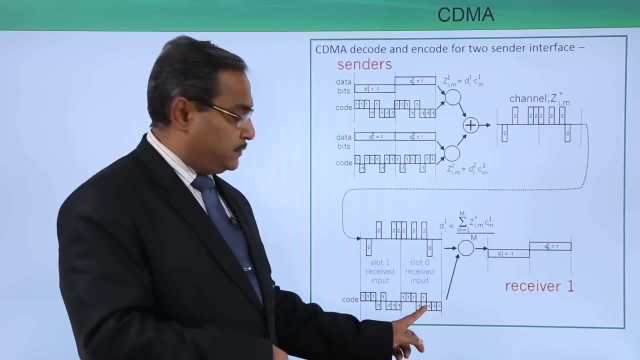 at its end. So see, here we are having 2 times 0. So these values will be ignored because if you go on multiplying they will be 0 minus 2 into minus 1, that is, plus 2, 2 into 1. that. 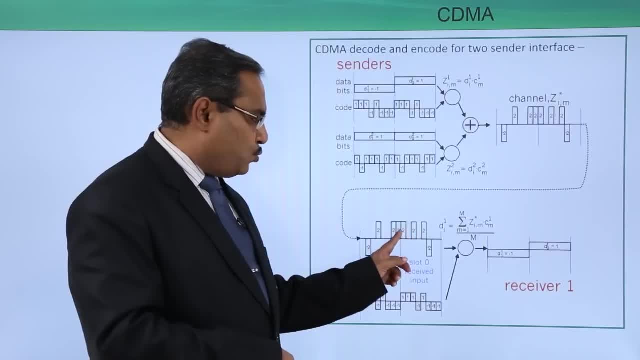 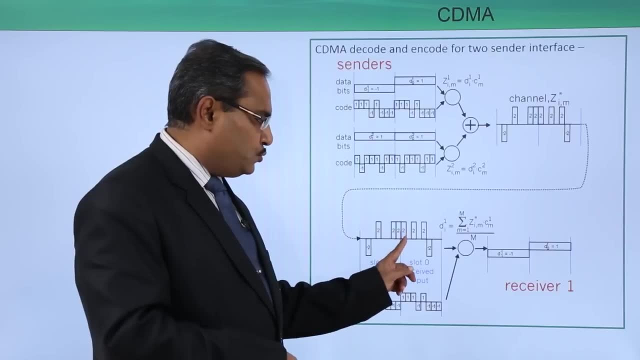 is plus 2.. So I have got 4. then we are having 2 times 1, 2 times 2 here and here we are having 2 times 1.. So in the next part we are having 0's. So 2 times 2 will be multiplied with 2 times. 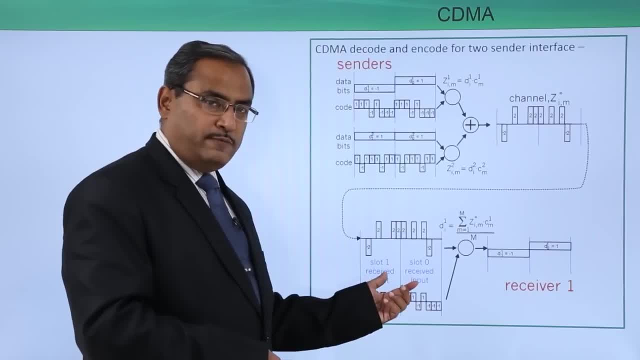 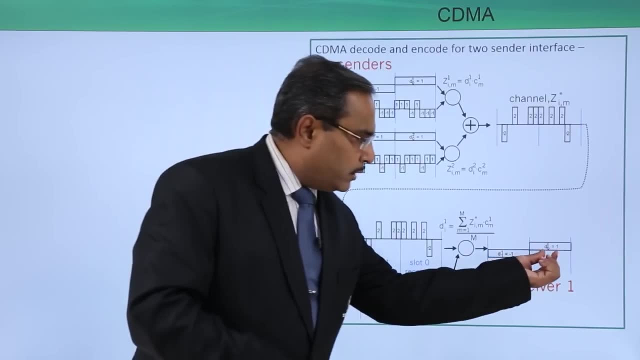 1.. So that will be 4. previously we are having 4.. So what is the total value? that is 8.. So what was the number of bits there in the code? 8.. So 8 by 8 it will be 1. in this way,